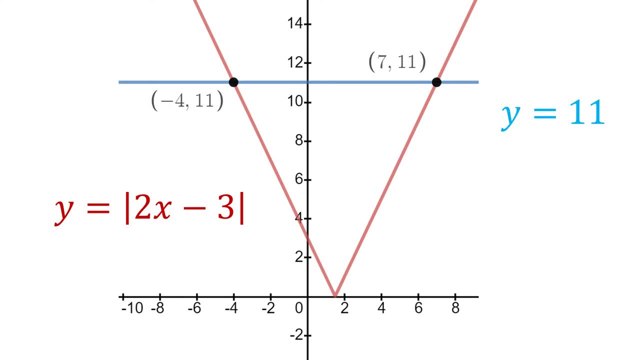 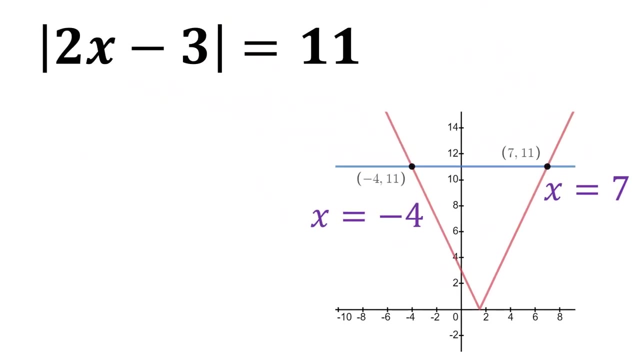 So what we actually care about graphically here are the x coordinates of those points of intersection. So we care about x equals 11.. We care about x equals negative 4, and x equals 7.. So, as we go back to that original equation, the absolute value of 2x-3 equals 11, what? 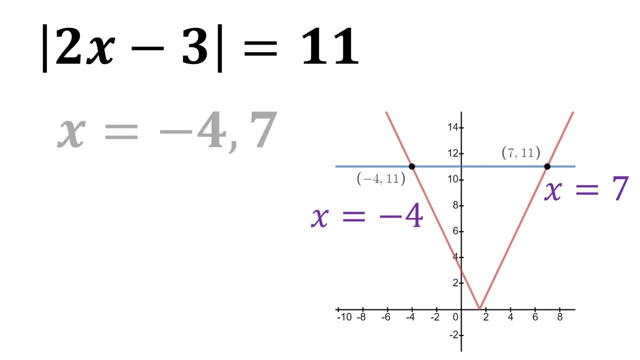 we can say about that now is that x equals negative 4 and 7.. And we'd solve this graphically by taking each side of the equation and graphing it on our coordinate system and seeing the points of intersection and just grabbing those x. 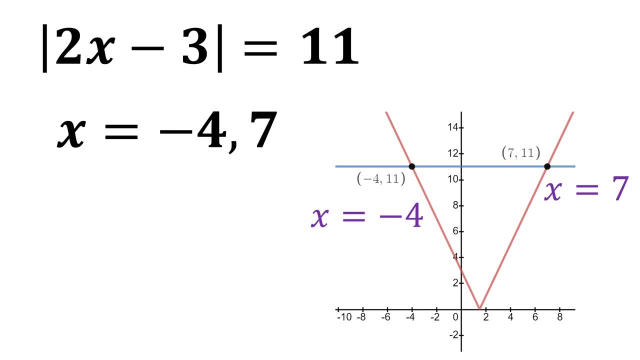 coordinates from those ordered pairs. And if you watched the first video you'll remember that x did equal negative 4 and 7 in that example when we solved it algebraically. So in this second example we have a little longer equation, we have negative 4 times. 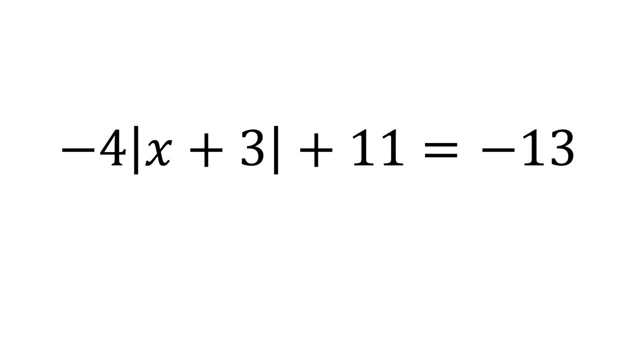 the absolute value of x plus 3.. We're going to add 11 to that and all that's going to be equal to negative 13.. So we're going to do the same thing, we're going to take each side of that equation and 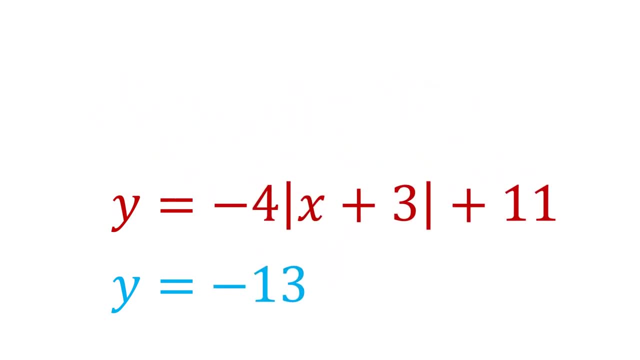 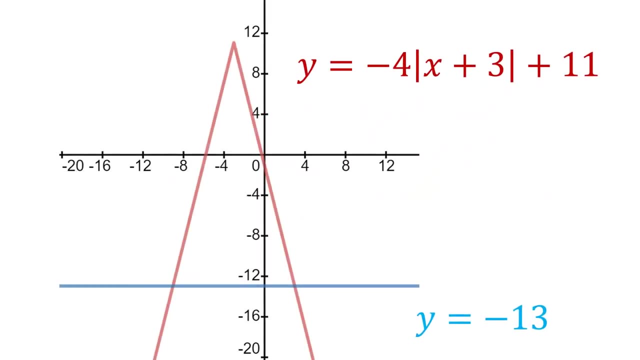 go ahead and put y equals, And so now we have two separate equations that we can graph. So we have the absolute value in red and we have our constant function here in blue, And once again you'll see there are two points of intersection and those ordered pairs will. 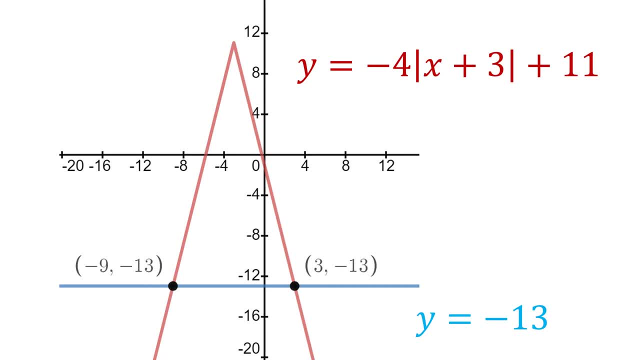 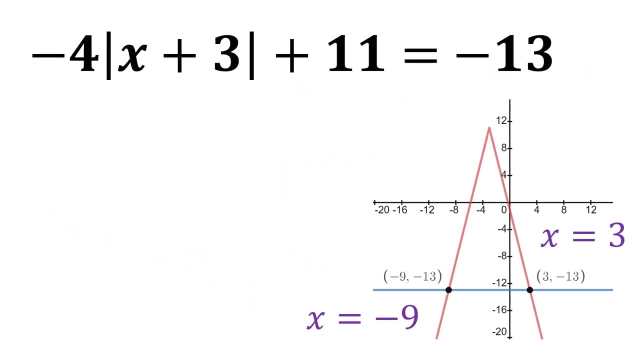 be negative 9, negative 13, and 3, negative 13.. So what we can take away from those ordered pairs are the x coordinates. So we have x equals negative 9 and x equals 3.. So when we go back and look at our original equation, what we can say is the solutions. 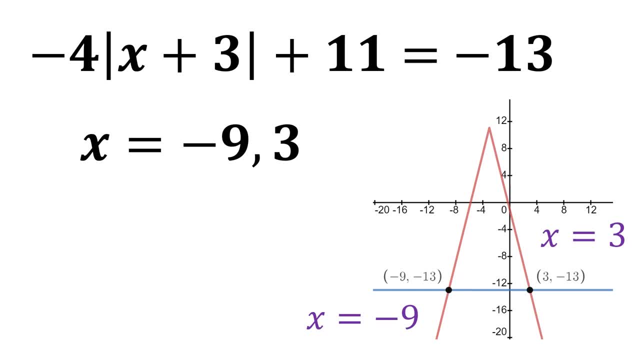 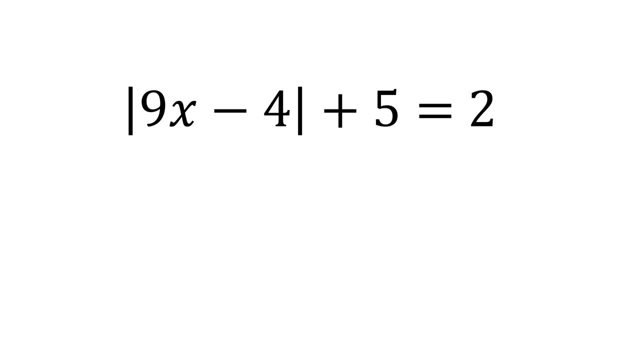 are: x equals negative 9 and 3.. And again, those are just the x coordinates of all the points of intersections. when I take each side of the equation and go ahead and graph them- And here's our third and final example- We have the absolute value of 9x minus 4, and we're going to add 5 to that and we're 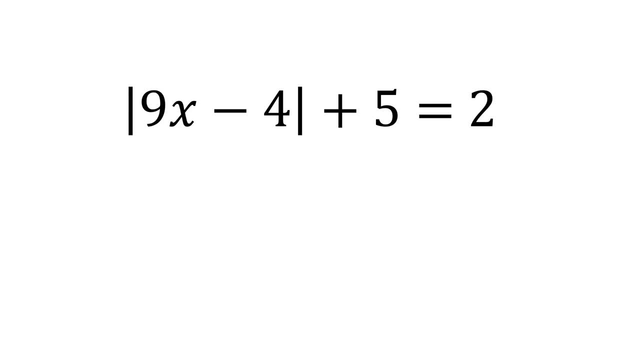 saying that equals 2.. So once again, we're going to take each side of the equation and set y equal to it, And so we have one in red and one in blue, and when we graph them it looks like this: 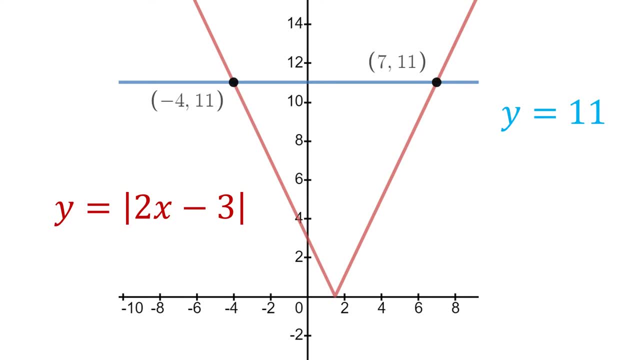 here are the x coordinates of those points, The points of intersection. So we care about: x equals negative 4, and x equals 7.. So, as we go back to that original equation, the absolute value of 2x minus 3 equals 11, what? 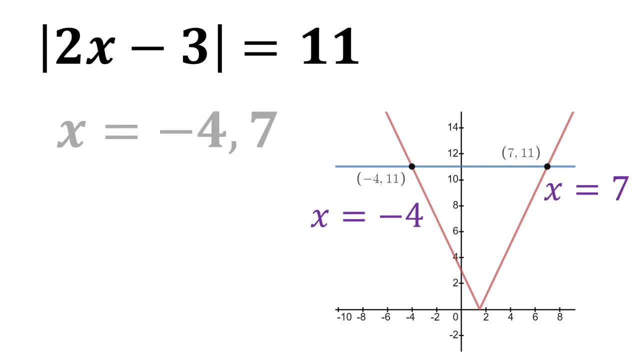 we can say about that now is that x equals negative 4 and 7.. And we'd solve this graphically by taking each side of the equation and graphing it on our coordinate system and seeing the points of intersection and just grabbing those x coordinates. 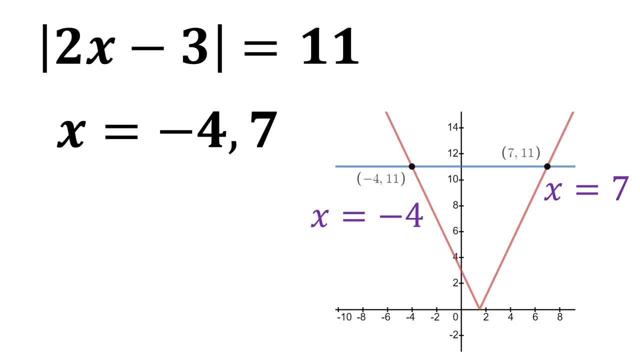 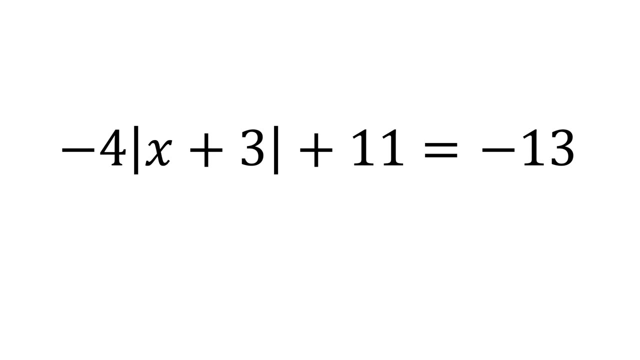 And if you watched the first video you'll remember that x did equal negative 4 and 7 in that example when we solved it algebraically. So in this second example we have a little longer equation. We have negative 4 times the absolute value of x plus 3.. We're going to add 11 to that and all that's going to. 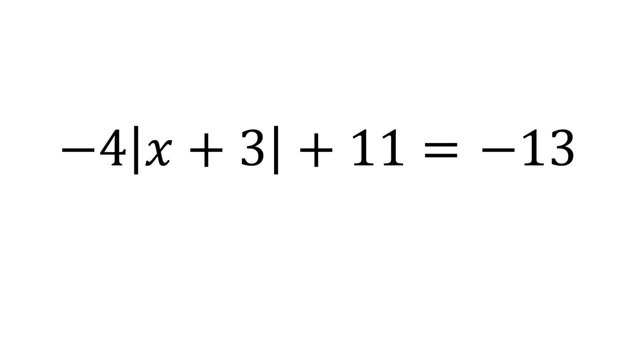 be equal to negative 13.. So we're going to do the same thing. We're going to take each side of that equation and go ahead and put y equals 7.. So we want to put y equals 7.. And so now we have two separate equations that we can graph. 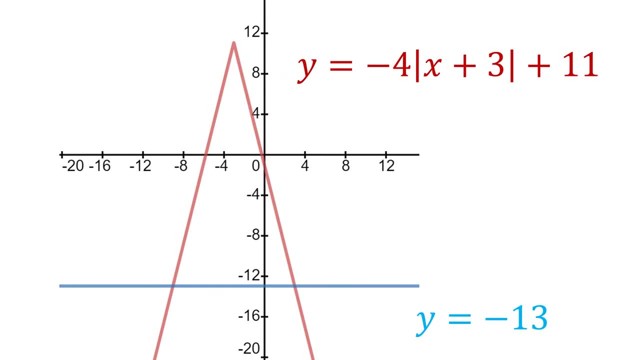 So we have the absolute value in red and we have our constant function here in blue And once again you'll see there are two points of intersection and those ordered pairs will be negative 9, negative 13, and 3, negative 13.. 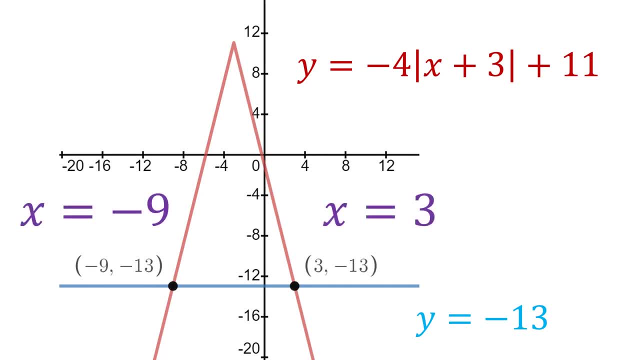 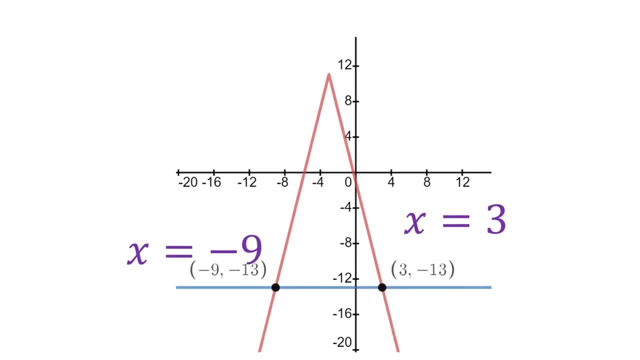 So what we can take away from those ordered pairs are the x coordinates. so we have x equals negative 9 and 7. and x equals 3. So when we go back and look at our original equation, what we can say is the. 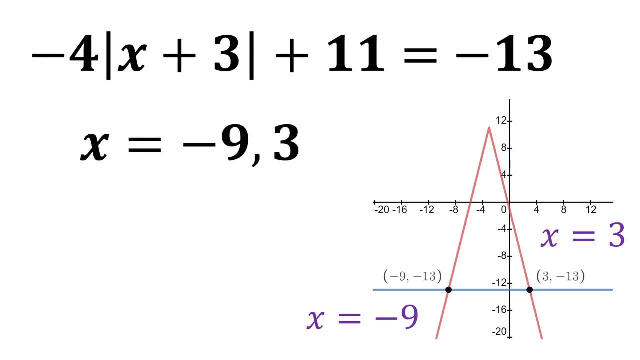 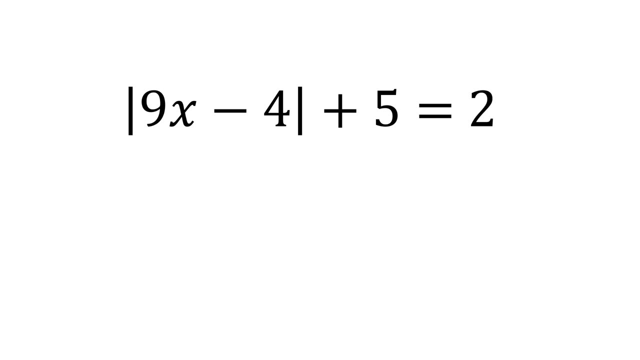 solutions are: x equals negative, 9 and 3.. And again, those are just the x coordinates of all the points of intersections. when I take each side of the equation and go ahead and graph them- And here's our third and final example- We have the absolute value of 9x minus 4, and we're going. 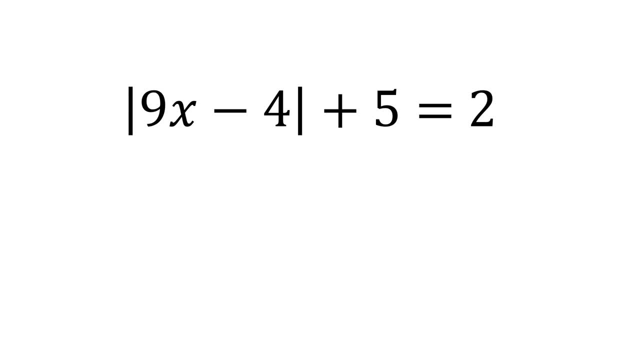 to add 5 to that, and we're saying that equals 2.. So once again, we're going to take each side of the equation and set y equal to it, And so we have one in red and one in blue, and when we graph,